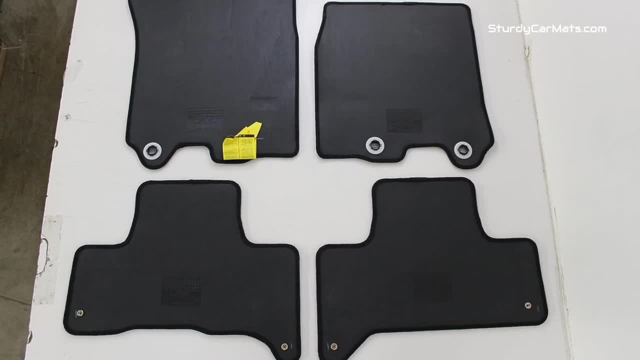 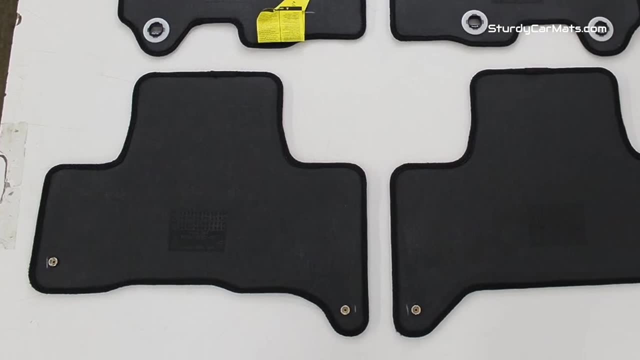 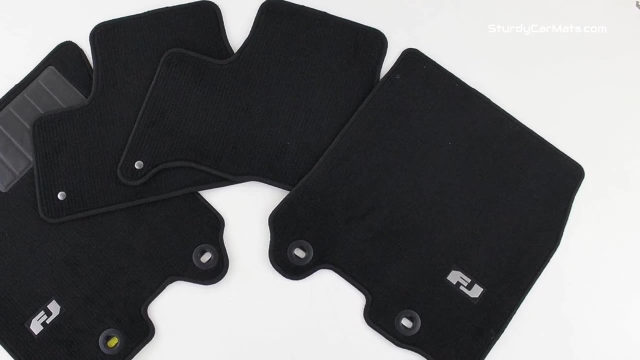 the customized design, you don't have to worry about the fitment anymore. Besides, this Toyota FJ Cruiser floor mat is made from eco-friendly TPE material. This mat is not only safe and odorless, but also highly durable and weather-resistant. As well as the rubberized 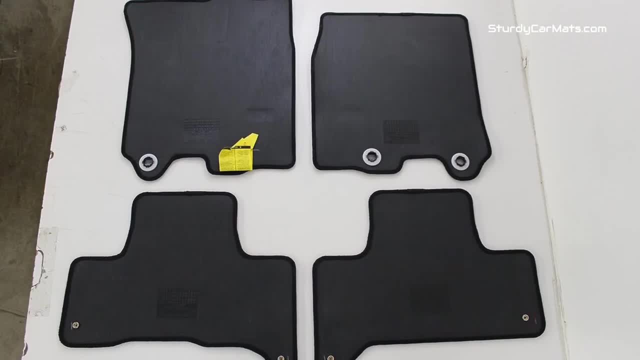 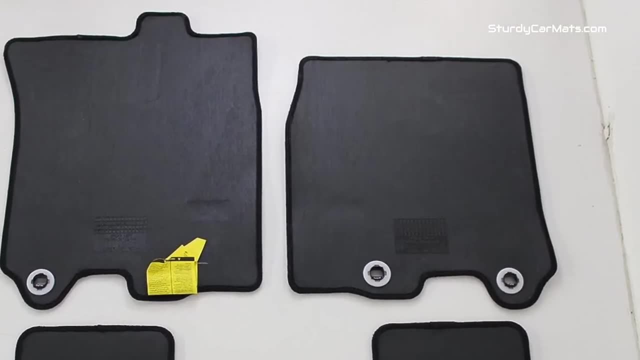 nibs on the bottom ensure a secure grip which prevents any sliding or shifting during the drive, And with their curly and raced edges, this mat effectively trap all kinds of spills, dirt and debris. that keeps your Toyota FJ Cruiser floor mat in good condition. 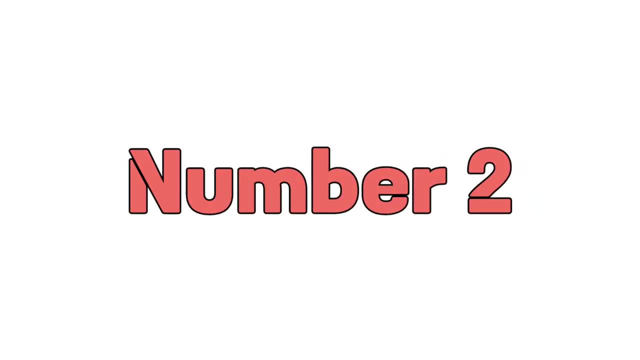 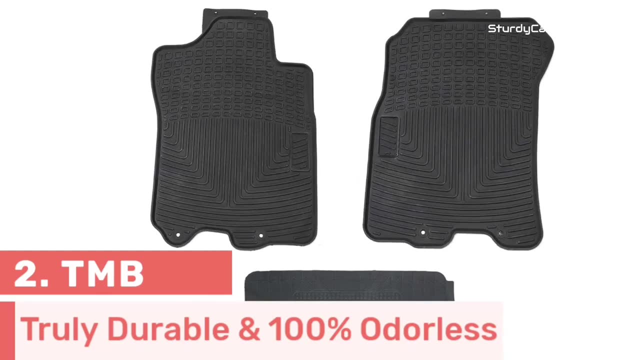 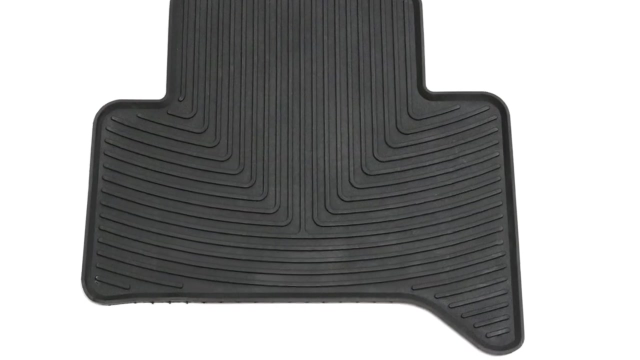 Number 2.. Now here comes the TMB floor mat for Toyota FJ Cruiser, and it is made of premium quality materials that provide the strength and durability for this mat. And this floor mat has custom design that ensures the perfect match for your 2007 to 2014 Toyota FJ Cruiser. 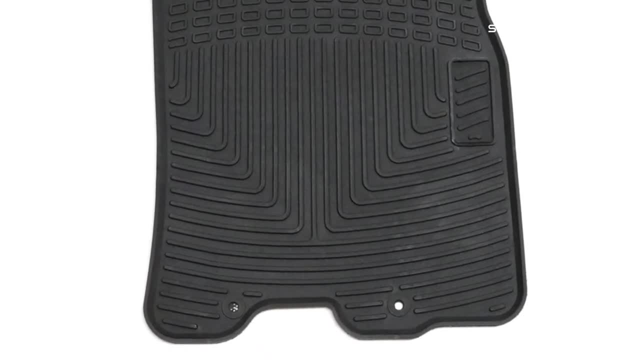 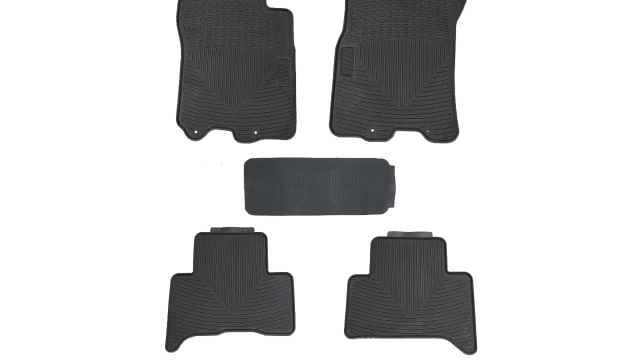 The curly and raised edges act as a barrier that can easily contain spillages within the mat, Which is why it prevents any kind damage to your vehicle's interior. Additionally, there are rubberized nibs are available on the bottom side of the mat. 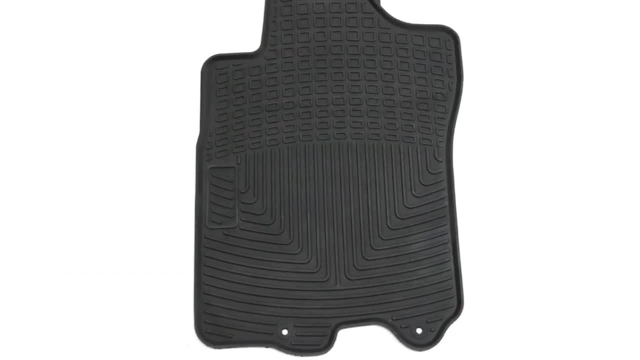 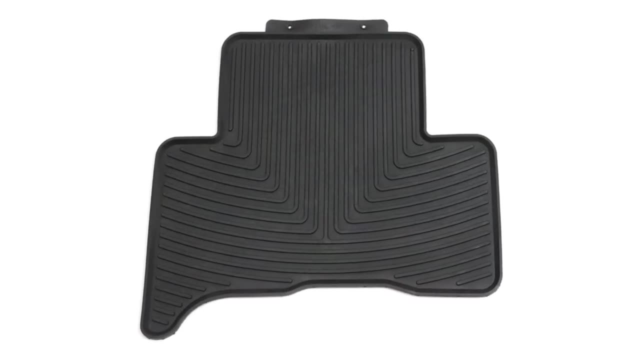 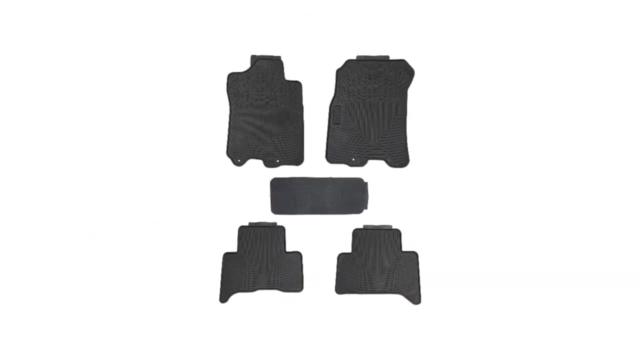 which prevents any kind of sliding and movement during the drive. Moreover, this Toyota FJ Cruiser floor mat is made from a 100% recyclable plastic rubber and polyethylene blend, which makes it truly eco-friendly and non-toxic car mat Plus. 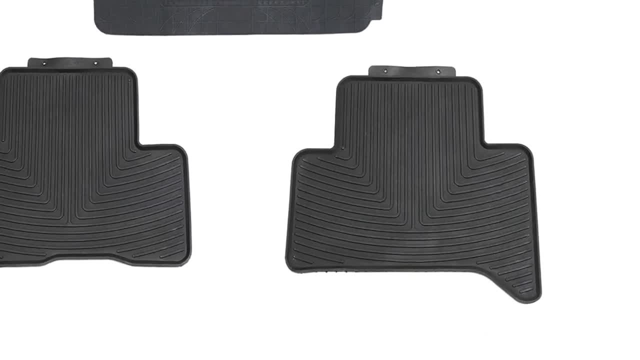 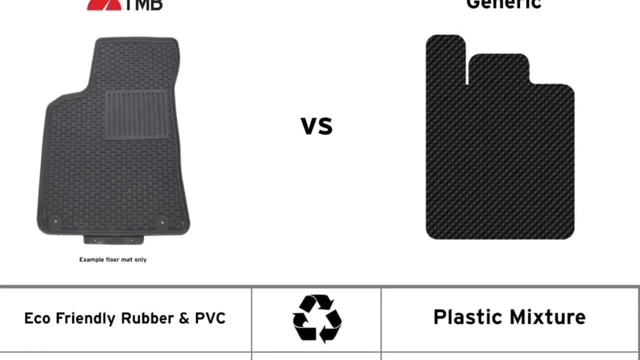 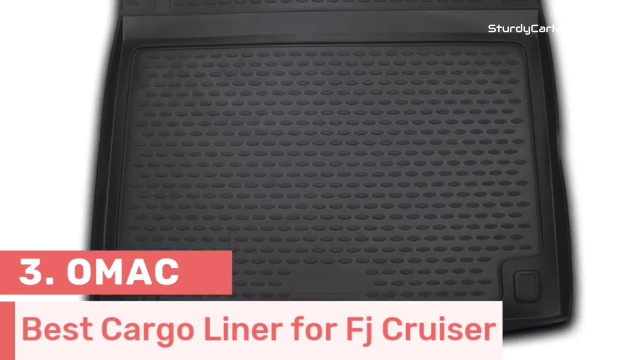 the all-weather protection offered by this floor liner makes it truly protective mat, as it protects your vehicle's carpet floor against snow, mud, sand and salt water. Number 3. The OMAC is the designer of these Toyota FJ Cruiser cargo liner that provides. 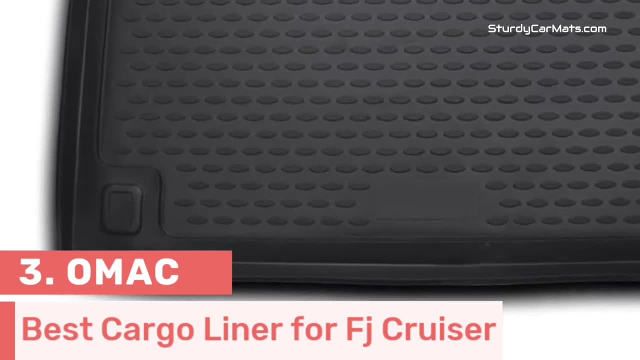 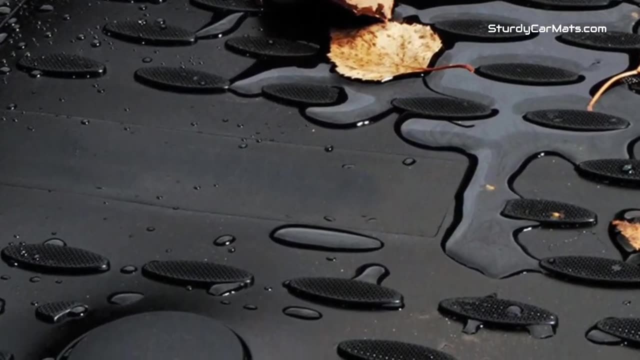 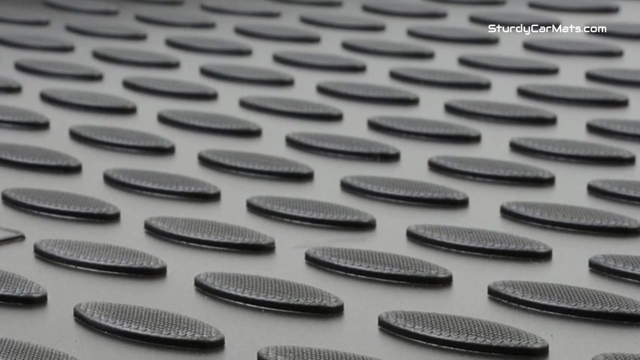 unbeatable all-weather protection for your vehicle, With a custom fit which is specifically designed for the 2006 to 2014 Toyota FJ Cruiser. that's why this mat provides a perfect edge-to-edge fit. Also, the rubberized nibs on the bottom side of the mat prevent any sliding or shifting. 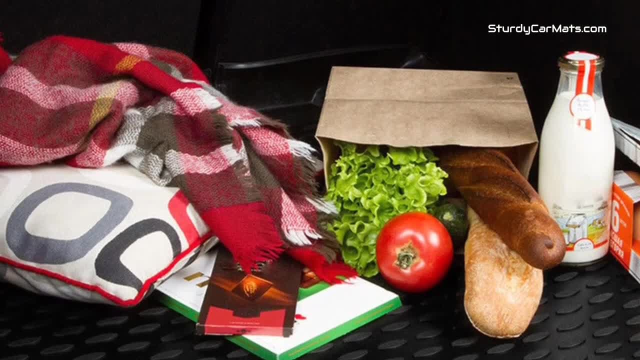 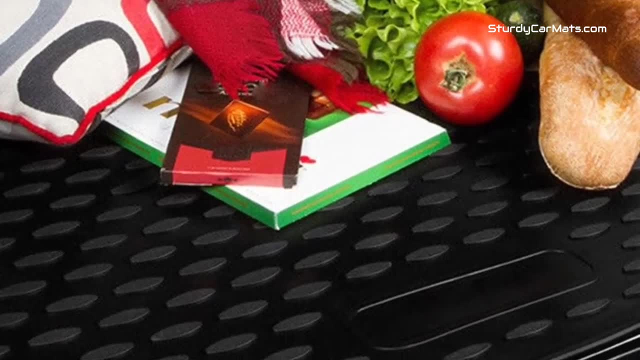 keeps them securely in place. Plus, the curly and raised edges act as a barrier and easily contain spillages and prevent them from spilling outside the mat. Furthermore, this Toyota FJ Cruiser cargo liner is not only functional but also easy to clean. 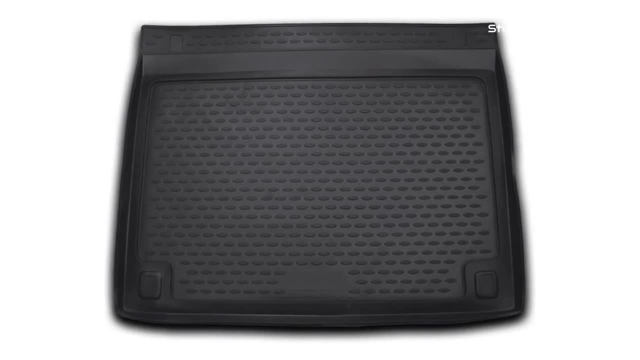 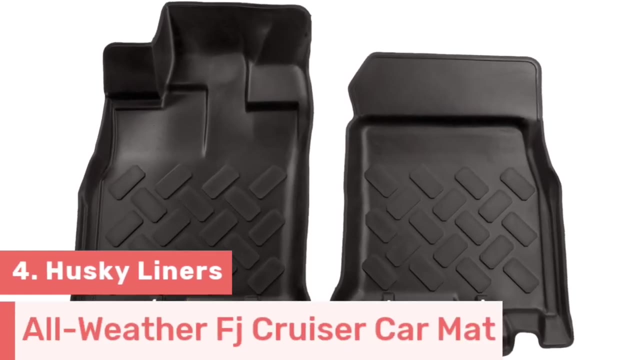 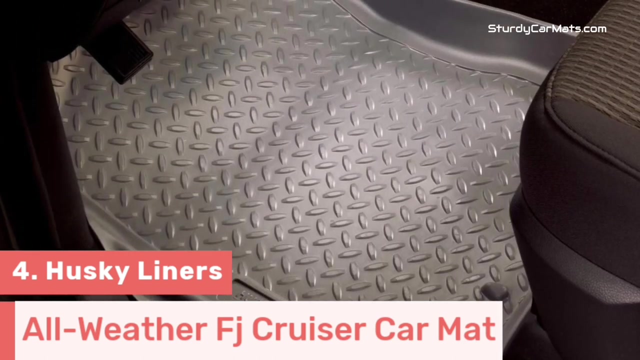 Simply remove them, hose them down and they're ready to go, making maintenance a breeze Number 4.. The designer of this first-row floor mat is Husky Liners, and it is a trusted name in automotive accessories. This Toyota FJ Cruiser car mat comes in a custom fit to ensure the perfect match for. 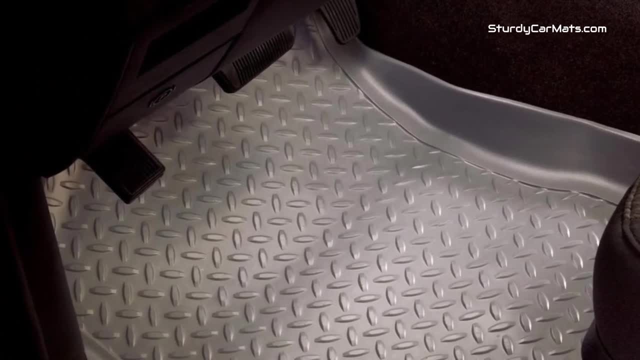 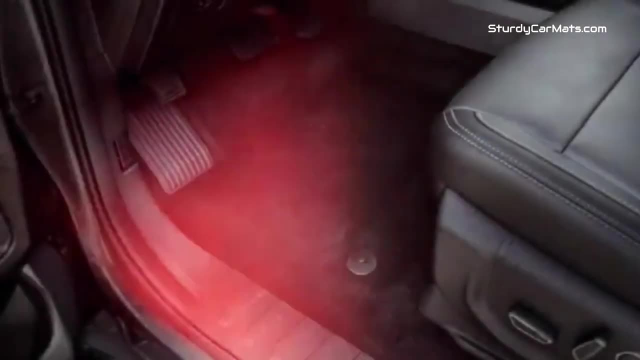 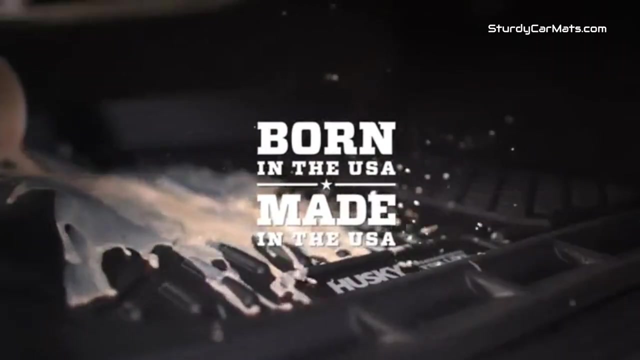 your 2011 to 2014 first row of Toyota FJ Cruiser, As well as the all-weather protection offered by this floor liner, makes it truly protective mat, as it protects your vehicle's carpet floor against snow, mud, sand and saltwater. Additionally, this Toyota FJ Cruiser floor mat is made from a. 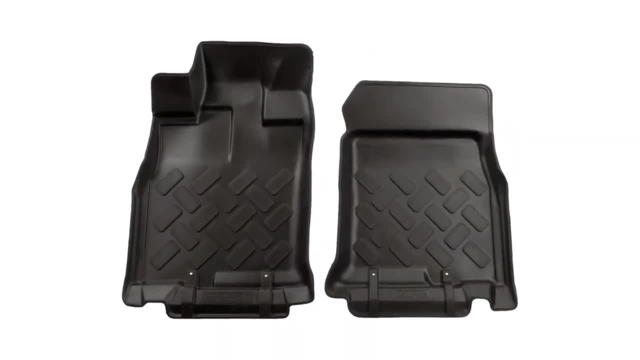 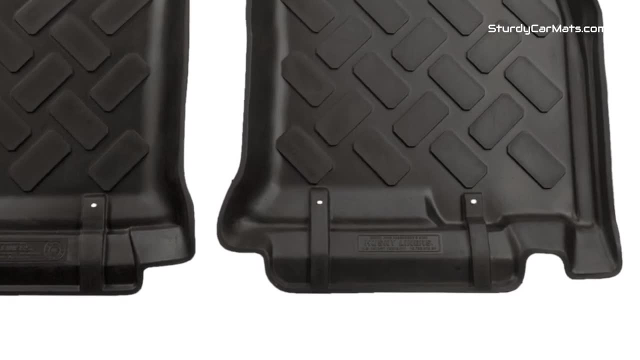 100% recyclable plastic, rubber and polyethylene blend, which makes it truly eco-friendly and non-toxic car mat. Furthermore, there are rubberized nibs are available on the bottom side of the mat, which prevents any kind of sliding and movement during the drive. 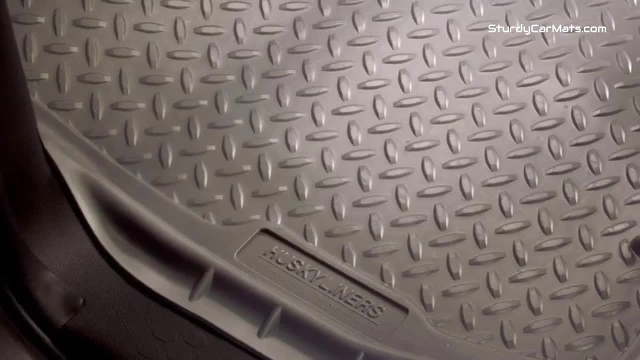 The curly and raised edges act as a barrier that can easily contain spillages and spillages. This Toyota FJ Cruiser floor mat is made from a 100% recyclable plastic, rubber and polyethylene blend, which makes it truly eco-friendly and non-toxic car mat. 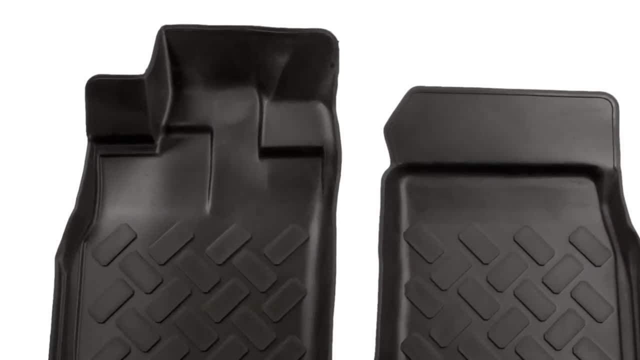 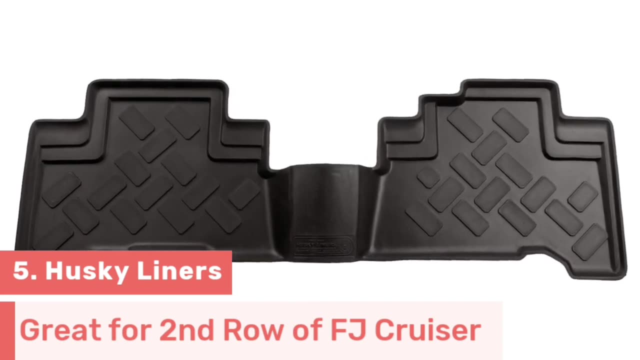 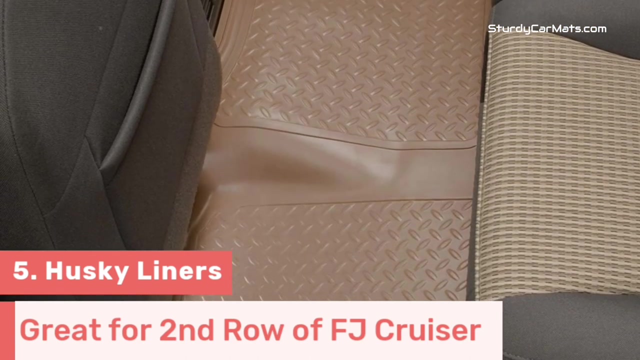 spillages within the mat, which is why it prevents any kind damage to your vehicle's interior. Number 5. Now here comes the Husky Liners again, but this time it is specifically designed for the second row of Toyota FJ Cruiser. With their all-weather design, they can withstand any. 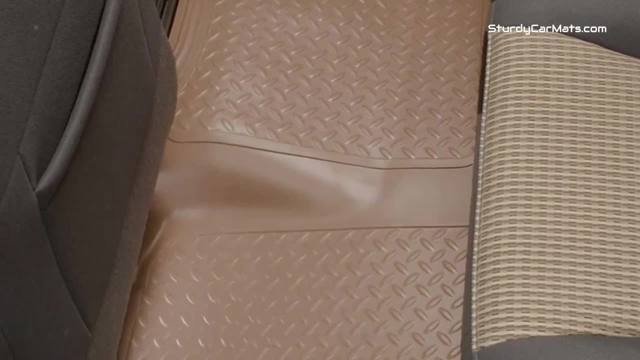 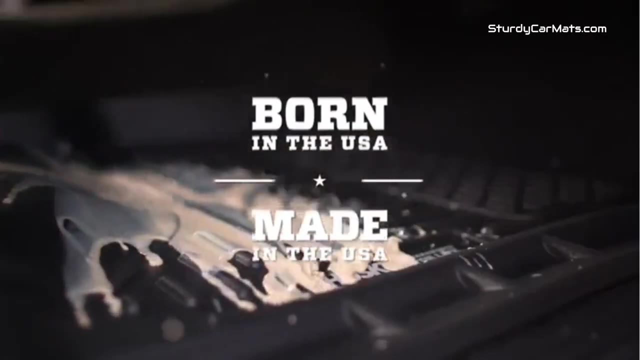 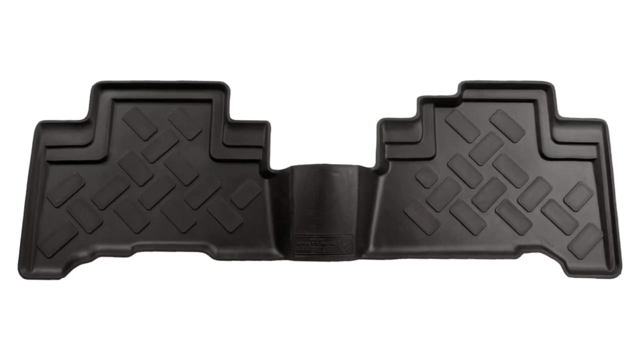 climate or season, like cold winter, hot summer and rainy seasons, as well as it ensures maximum protection against dirt, mud and spills. As well as this, Toyota FJ Cruiser floor mat offer very high quality and functionality to enhance the interior of your vehicle. 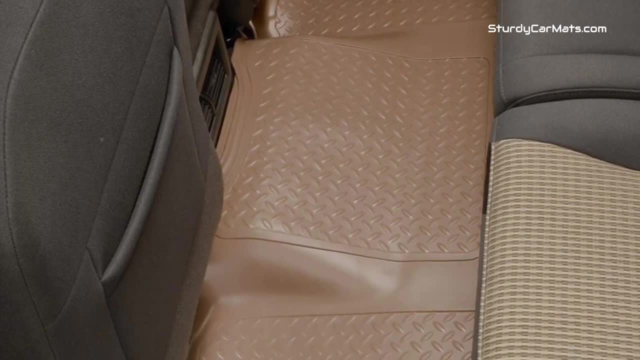 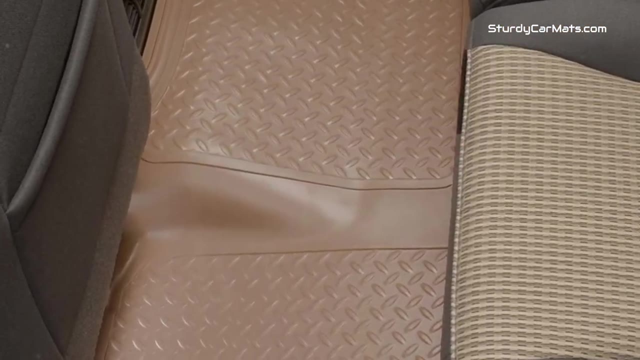 thanks to the rubberized nibs on the bottom side of the mat, as you can be sure about the sliding or shifting while driving. Moreover, the curly and raised edges of this mat effectively contain any spillages, which keeps your vehicle's floor free from damage.